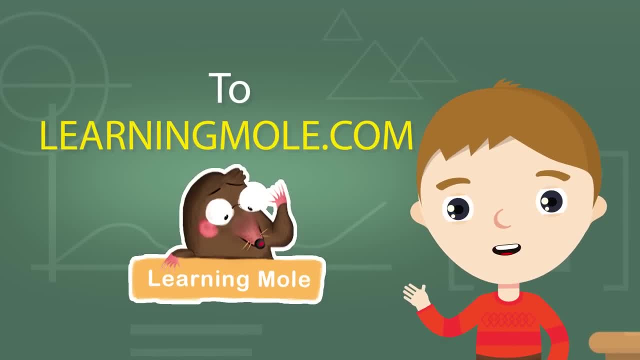 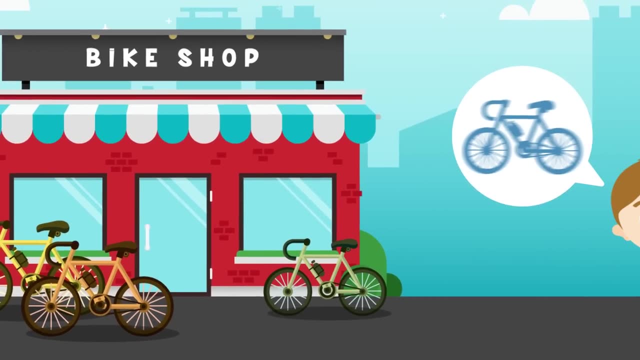 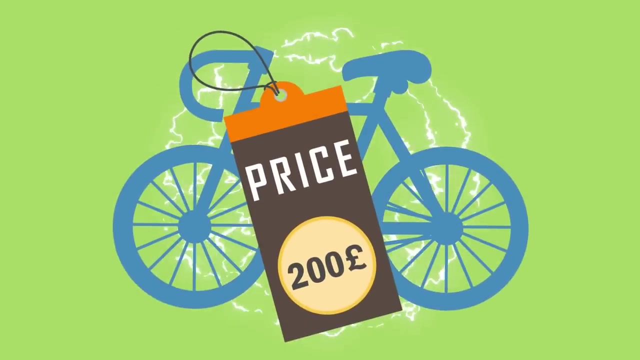 Welcome to learningmallcom. Today we're going to talk about earning money. I asked my dad to buy me a new BMX bike. It's amazing. You can do all sorts of tricks, but it is a little bit expensive. Guess what my dad says. when he saw the price, He said: 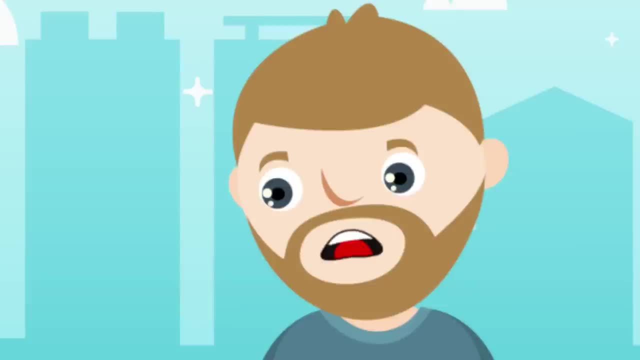 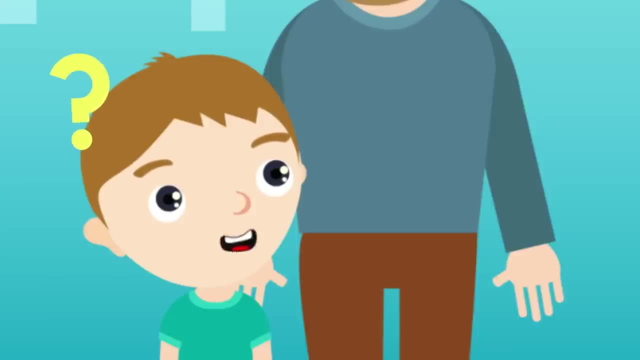 Aaron, I will pay half, but you will have to save the other half. That's nearly a hundred pounds. I said I never get that much for my birthday And he just replied: Well, you're going to have to earn it well, aren't you? 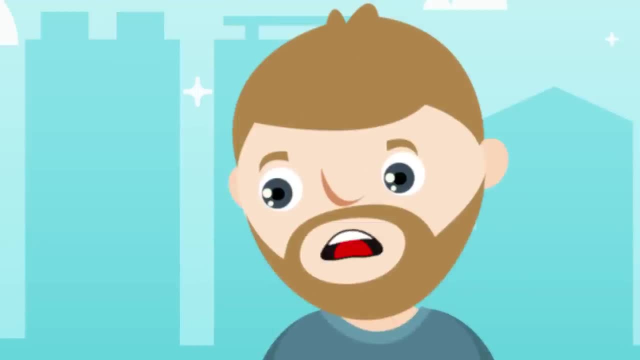 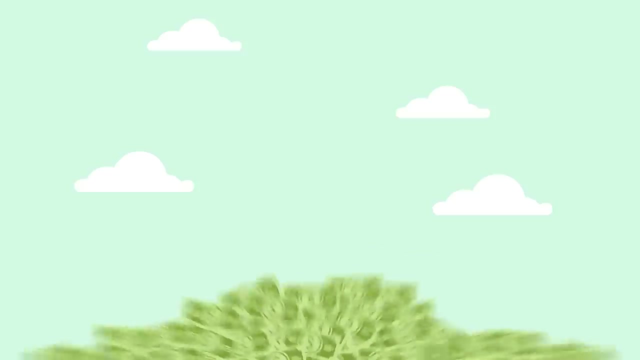 Earn it. What do you mean, I asked? Well, my dad said you'll have to do some work in order to earn money to help pay for your new bike. He then went into a long story about the olden days, Apparently. 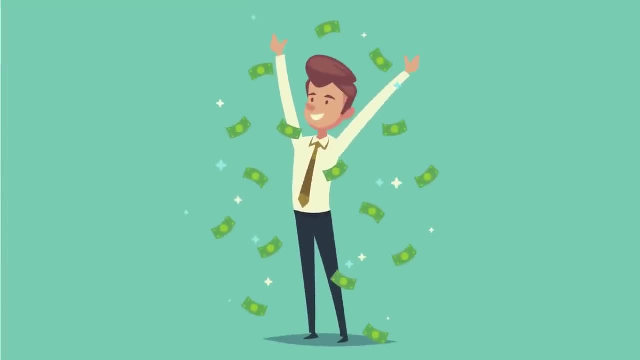 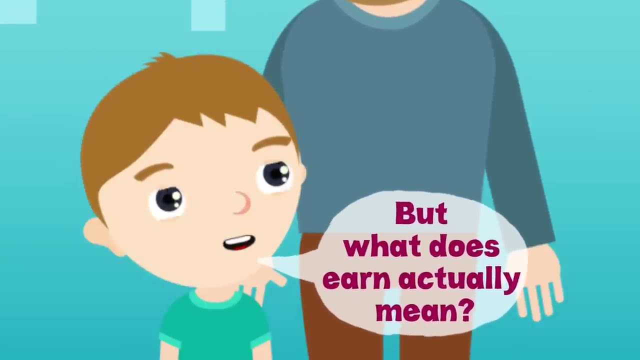 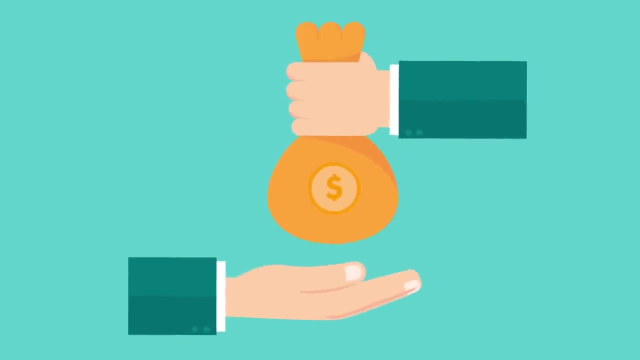 money doesn't grow on trees or disappear in people's bike account. You must earn it. But what does earn actually mean? Well, you work, do a job or provide a service and someone will pay you money in return. So basically, if you work, you can earn money. 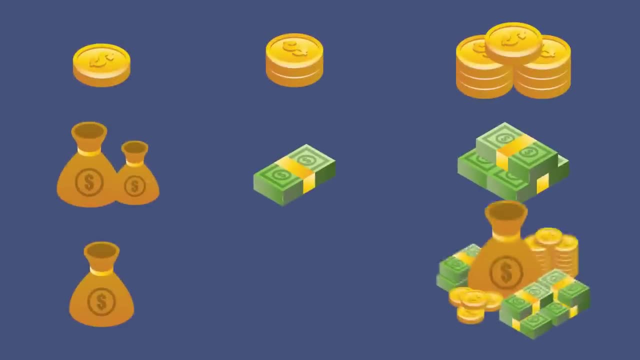 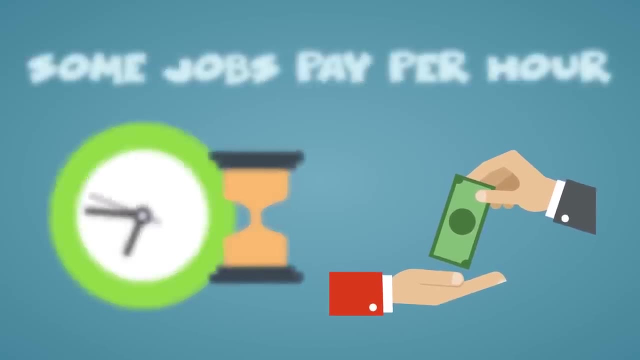 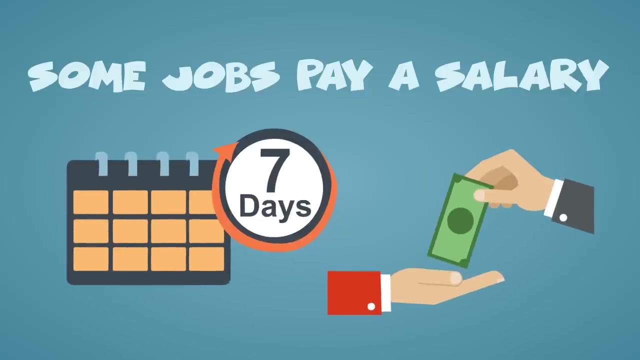 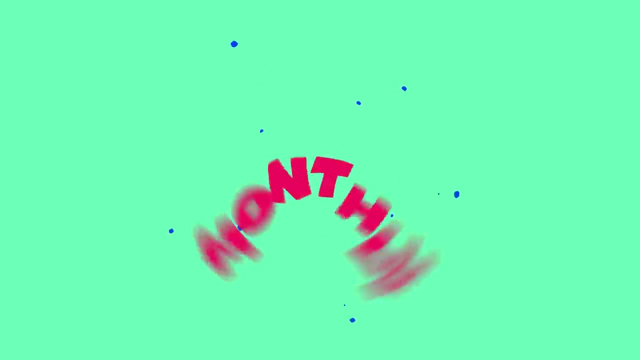 Different types of jobs pay different amounts of money. Some jobs pay pay per hour, So the more hours you work, the more money you earn. Some jobs pay a salary. This means you must work a certain amount of hours each week to earn your salary. Depending on your job, you can be paid daily, weekly or monthly. 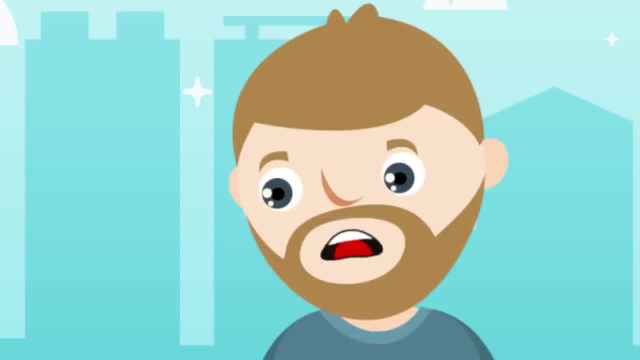 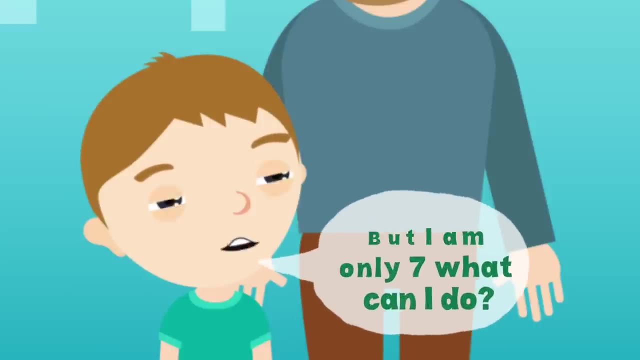 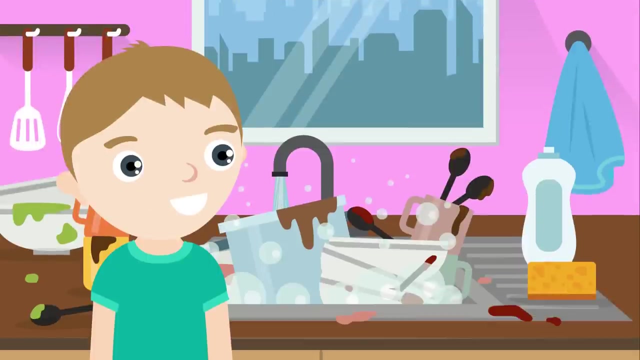 So after the longest explanation in the world, I finally understood I will have to do some work to earn some money. But I'm only seven. What can I do, I said. Then my dad produced the list: Help with the dishwasher, Help wash the car, Help your granny with her shopping Tours all around the 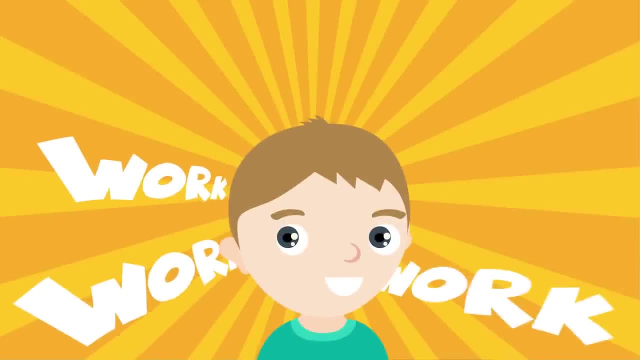 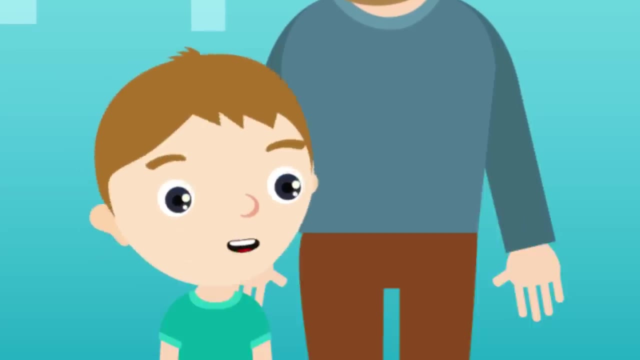 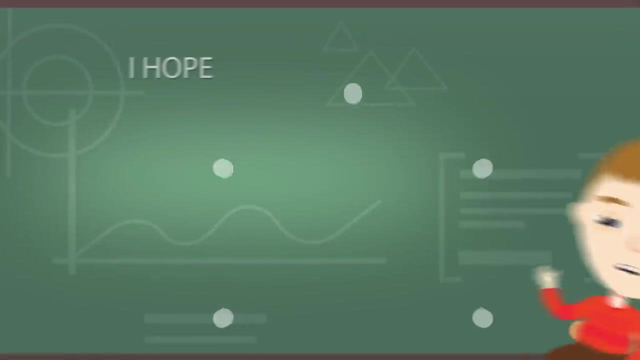 house. The list kept going and going and going. There are loads of jobs that you can do. My dad said I really don't mind doing some work if I can earn money to get my BMX, BMX bike a little bit quicker. I hope you enjoyed my story, but I must get going and